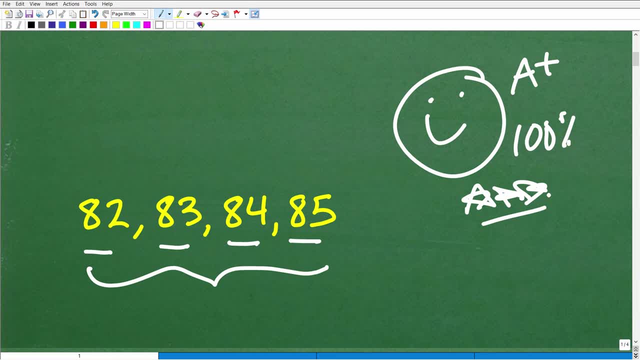 know what. I know how to solve a math word problem involving consecutive integers. They're just going to be flabbergasted with that information. They're going to be like, wow, you know, very impressive. Okay, so let's get into the problem, and the first thing we need to understand is: 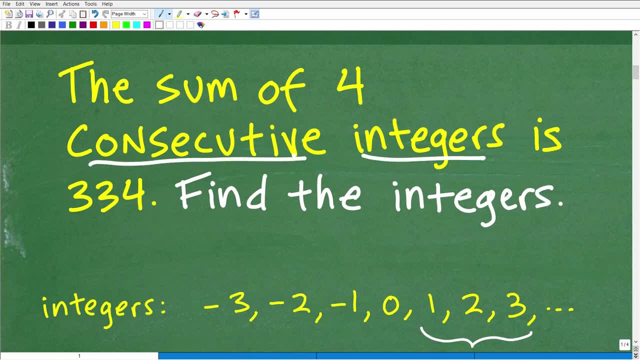 this word integers and this word consecutive. Okay, so of course you know. if you're like, I'm not sure what the word consecutive means, well, you're going to be confused on what to do. So let's talk about integers and consecutive integers. So, basically, 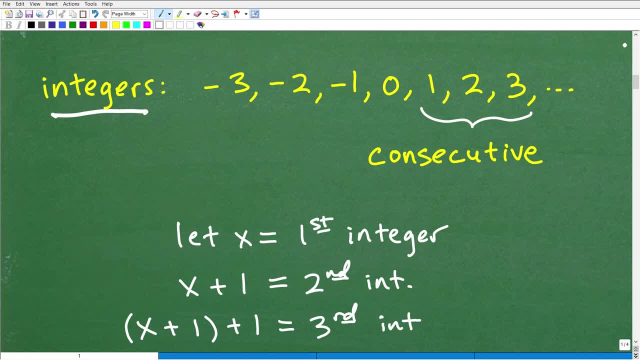 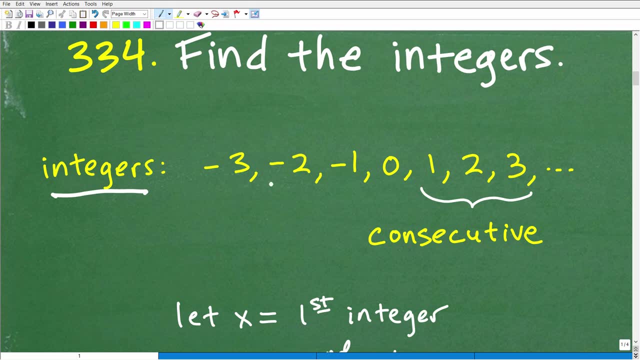 here are integers. Okay, now, integers are a type of number. Okay, there is a subset of the real numbers. Okay, so negative, three negative two. negative one, zero, one, two, three. these right here are what we call integers. Okay, on the real number line. Now, hopefully, 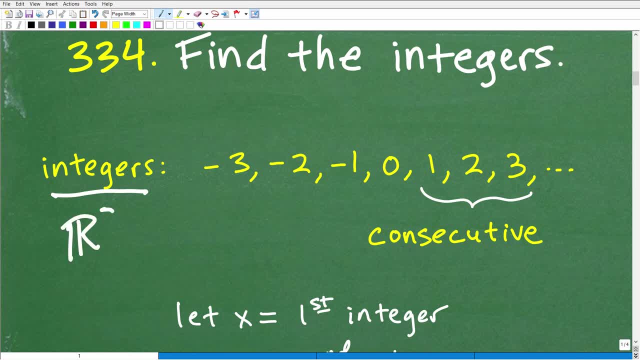 you remember that. And again, this is part of the real number set. Okay, it's a subset of the real number system, But numbers like this, which are whole numbers, right, these are one, two and three. These are what we refer to as natural numbers or counting numbers in mathematics. 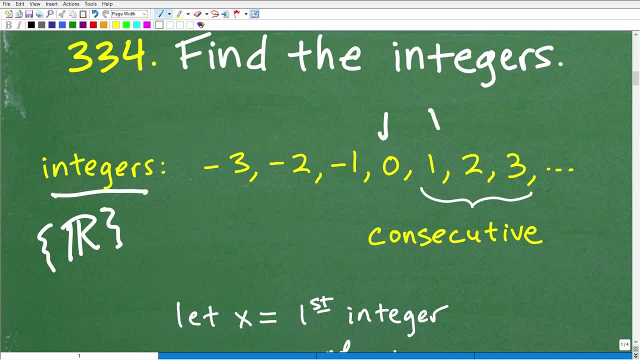 Then we throw in zero, we have the whole numbers, And then here these are the positive whole numbers, And if I have the negative, I have the positive whole numbers, And if I have the negative negative whole numbers, this entire set here is a set of integers. Okay, but I don't think it's. 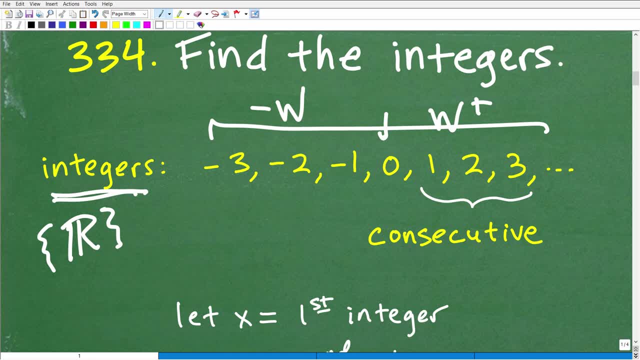 really you know. ultra critical that you remember all of this. you should know the different type of number systems. Okay, that's really important. But if you kind of forgot the specific definition of an integer, as long as you recognize integers as these type of numbers, then you're good to go. 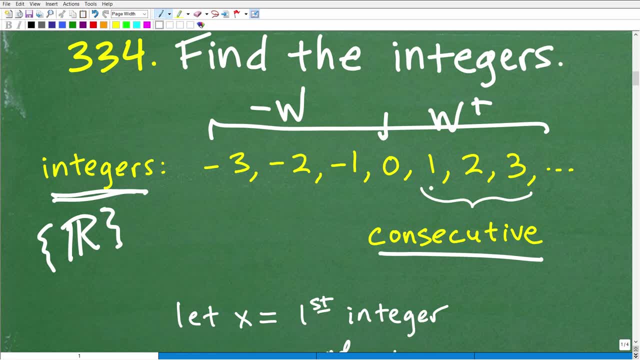 Now let's talk about the word consecutive. Consecutive just means, if I said, three consecutive number right after another number. So, for example, one, the next number is two, the next number is three. these are three consecutive numbers. Okay, so things like four, seven and nine. these are 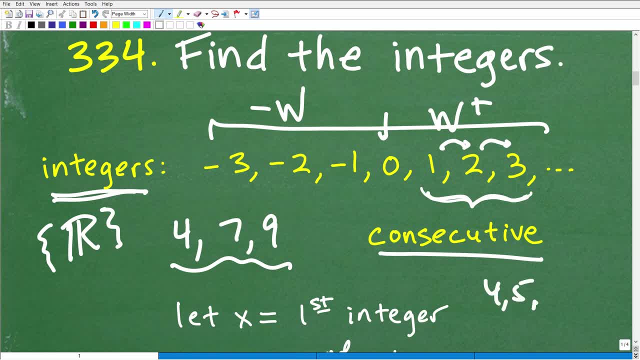 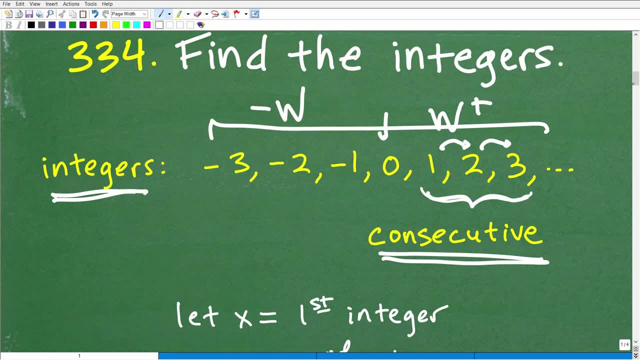 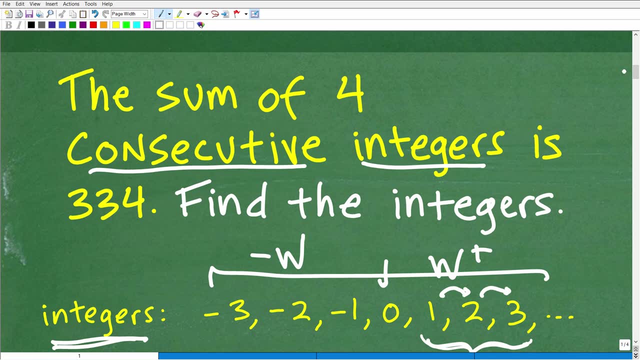 that what we need to do is go back to the problem, because we are dealing with a math word problem And you always need to read these things at least a couple, two or three times at a minimum. Okay. so the first time I read it I'm like, okay, I got a sense of the problem. The second time I read it, 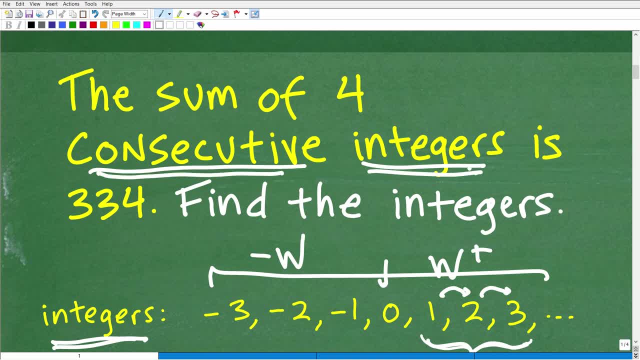 I'm like: all right, I need to understand what consecutive an integer is, And I know I have four, okay, four numbers that add up to 334.. And these four numbers happen to be integers and are also consecutive, meaning they're going to be coming. 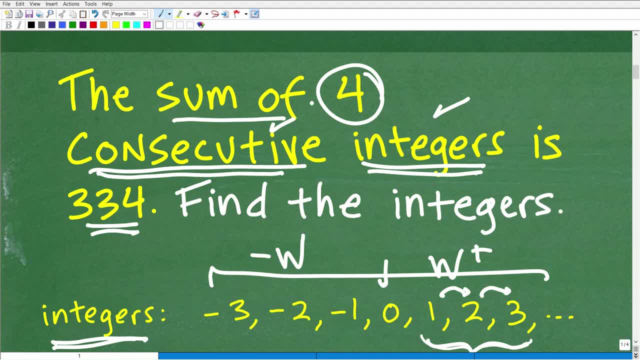 they're going to come right after another. Now I can imagine maybe some of you that were like. you know, I could kind of just test the waters. I got 1234, I add all that up. These are four consecutive integers. it doesn't add up to 334.. And you just keep playing with consecutive. 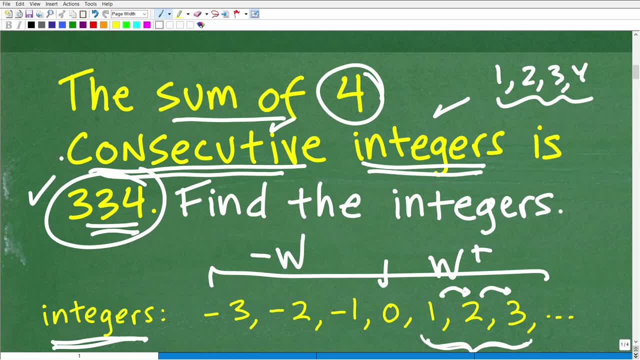 integers until you, you know, through trial and error, to your finest, but that would be the long way. What we want to do here is construct an equation To solve this, And this is a very common type of algebra word prompt. So let's go ahead and get. 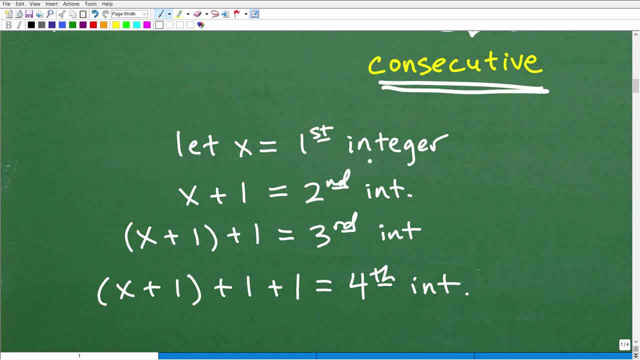 into this right now. So we're going to let x equal our first integer. okay, we're going to establish this variable x as our first integer. whatever that might be, all I know is that if this is x, the next number right after it is x plus one. okay, And I need the number right after x. 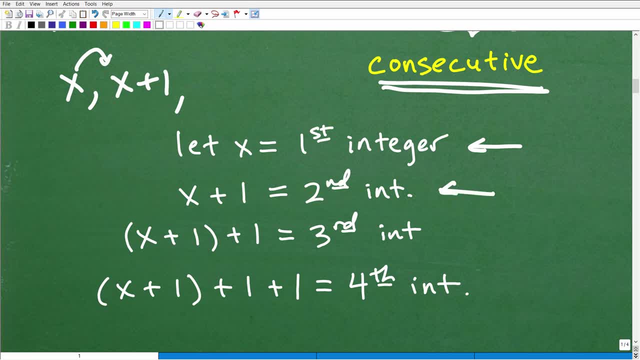 because we're talking about consecutive numbers. So our second integer would be x plus one. And then, if I take x plus one and add a one to it, this would be my third integer. x plus one plus one or x plus two. right, that would be my third integer. And then, of course, 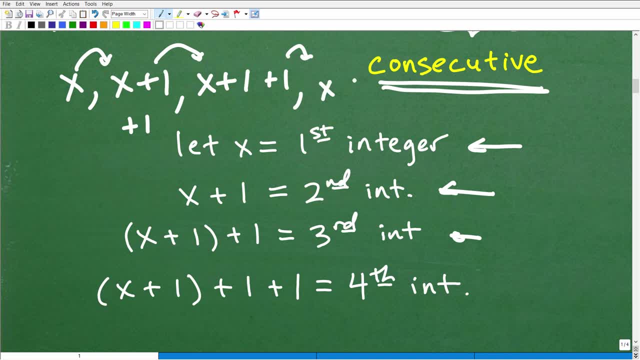 if I add another one to it, so I get x plus one plus one plus one or x plus three. this right here would be my fourth integer, 1234.. So I can model these mystery integers right here And these would be four consecutive. 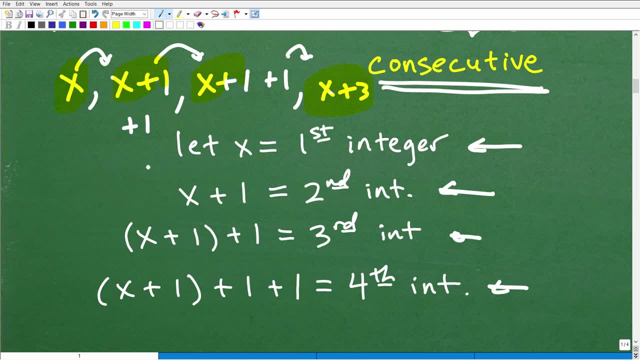 integers and I don't know what the actual values are, But certainly from an algebraic standpoint, I can kind of write this model out. And that's what you need to do, And you know when you're solving a problem like this- is to pick a variable okay, and you need to define. 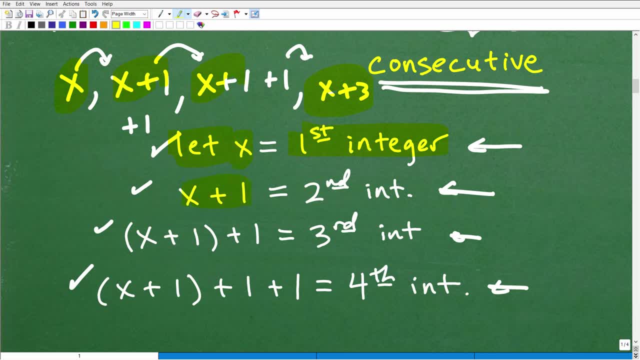 what it is. you're letting x equal the first integer, x plus one equal the second, and so forth. All right, So hopefully you know, you understood that, because you understood what the concept of consecutive is. So let's go ahead and get started. So let's go ahead and get started. 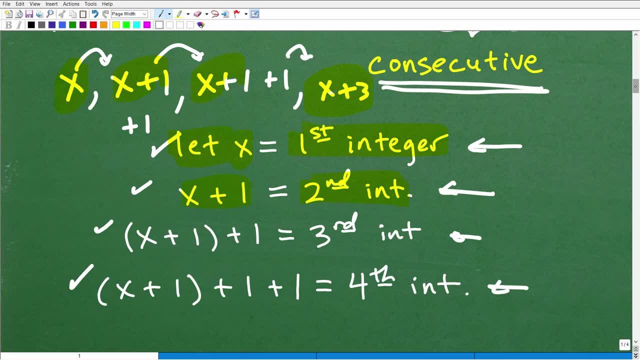 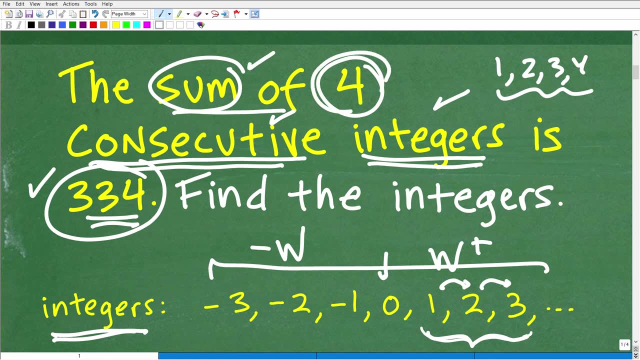 But now what we need to do is like go back to the problem. Okay, we're like, all right, what does the problem says? The problem says what the sum, the sum, In other words, if we add up these four consecutive integers, you're going to get 334.. So that's what we're going to do. 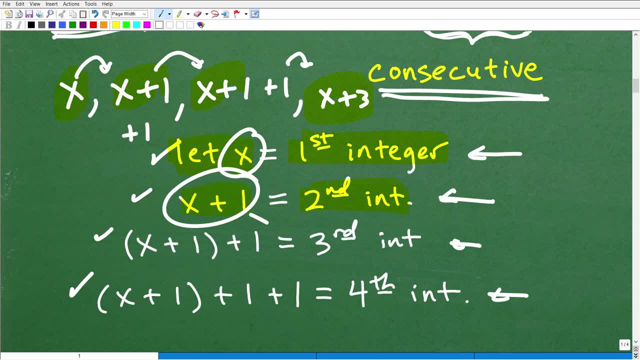 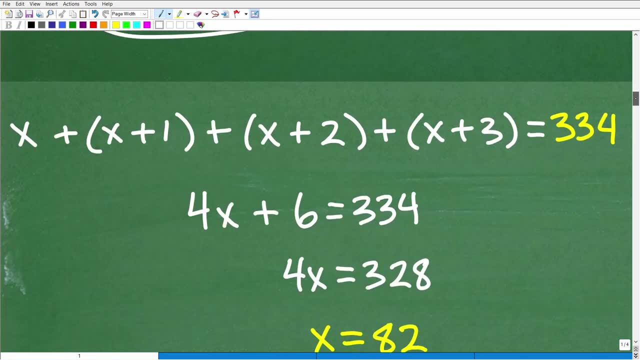 We're going to take these four integers here- 1234, four consecutive integers- And we're going to create an equation. We're going to add those up because we know the answer is going to be 334.. So here's our first one. 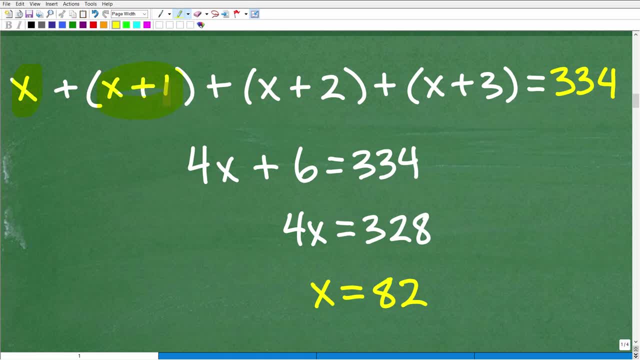 x plus one is our second consecutive integer. And then we add another one right to this, plus one. x plus one plus one, That's x plus two. That's our third. we add a one to this, that'd be x plus three. 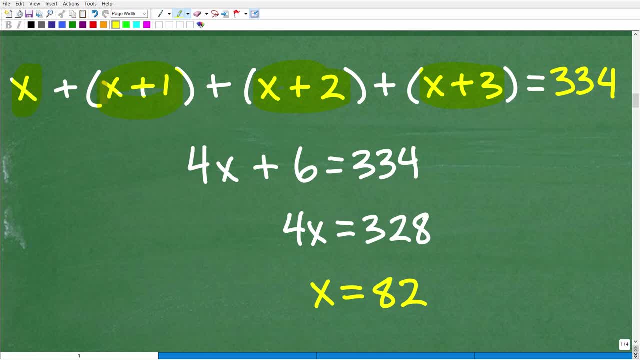 that's our fourth. So these are our four consecutive integers. the sum of our four consecutive integers is equal to 334.. So now all we need to do is solve this lovely equation for x. So we have x, x, x and x. that's four x, right? So four x's, then we have one. 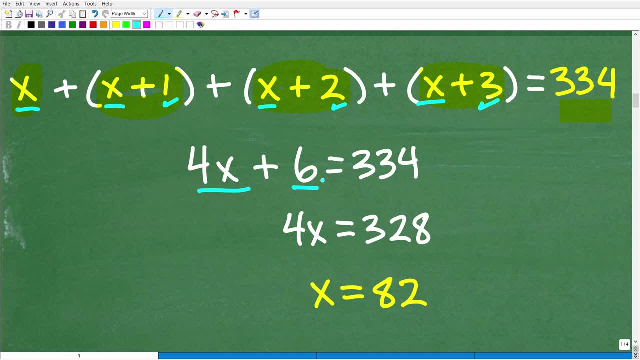 and two and three, that gives us six, And so we're just doing some basic algebra here. So let's solve for x. What we need to do now is: subtract six from both sides of the equation. I get four. x is equal to 328.. And now I divide both sides of the equation by four. 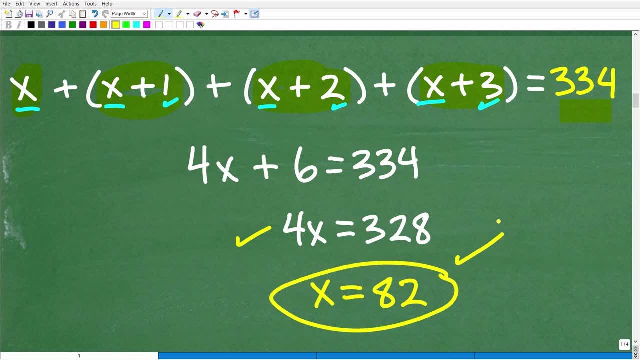 I get x is equal to 82. So what is that? Well, that is our first integer. okay, And we know that we have four consecutive integers. if it starts with 82, let's just use common sense- Well, okay, 82,. the next one, it's gonna be 83,. the next one is gonna. 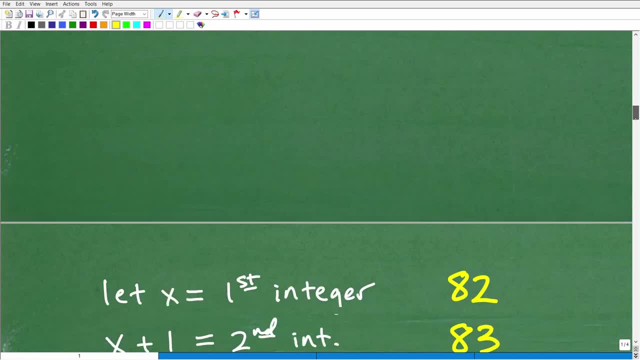 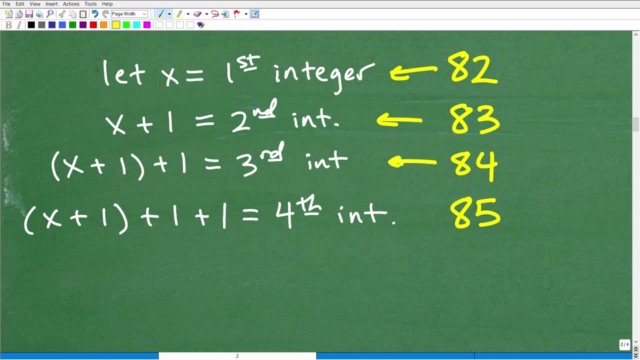 be 84, etc. etc. But if you were kind of confused about that you could just go back to our little model here. x was equal to 82, x plus one, of course, 83, x plus two from from our 82 is 84..